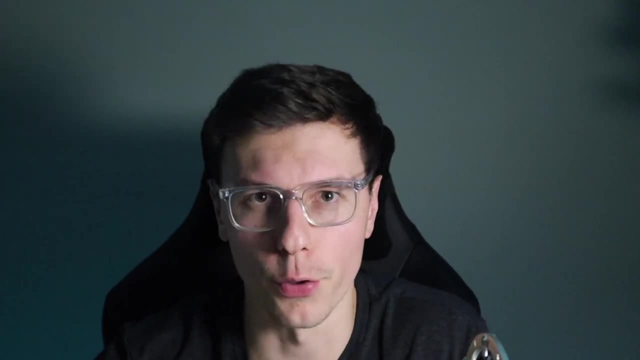 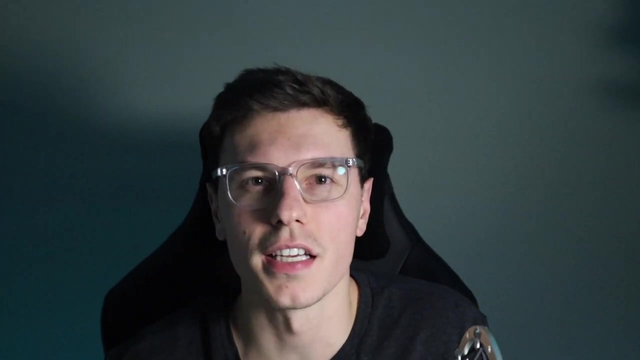 So I wanted to quickly cover the difference between imperative and declarative programming. This was something that took me some time to understand, So I figured I would explain it to you quickly. So the most common definition you'll see is that imperative programming shows you how. 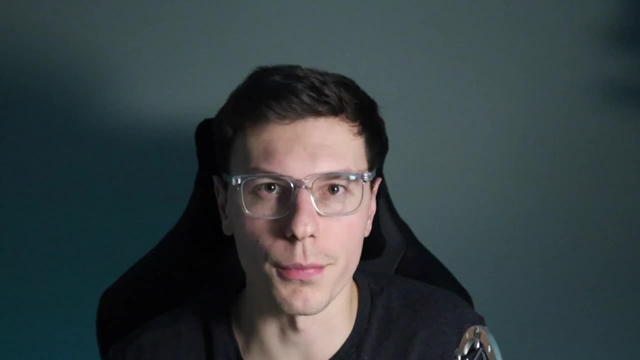 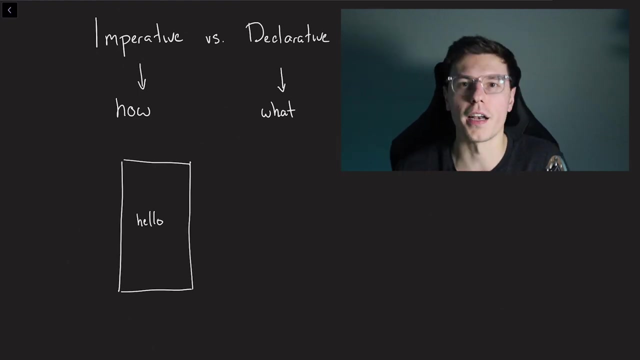 to write code and then declarative shows you what you want to get from the code. Now this kind of confused me for a little bit, So I want to show you an example. Let's pretend we have an app that says hello, in the middle of the screen. An imperative solution would be for the code to 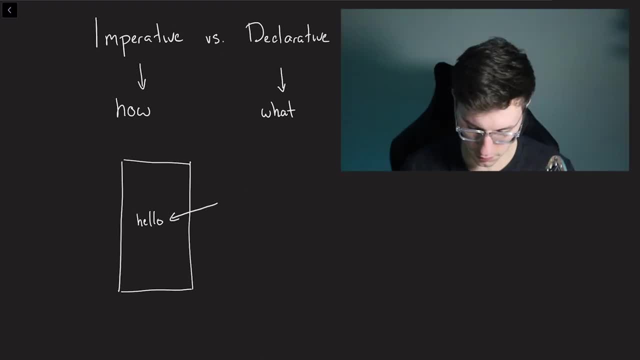 tell the app to go change that text. So basically you go in and maybe have a function called set text and it takes that text and changes it to whatever else you want. Now a declarative solution is completely different. A declarative solution pretty much tells a state that it wants to see a 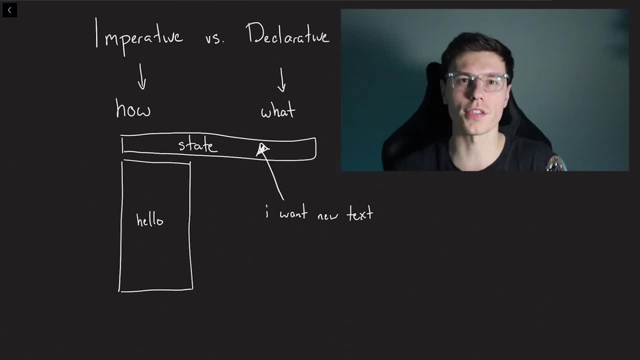 different text, Then it will update that state. The state causes a rebuild and then on the screen you should see your new text. The difference is imperative is actually describing to the app, or to whatever, what you want to do. You want to see your new text and then on the screen you should see your new text. 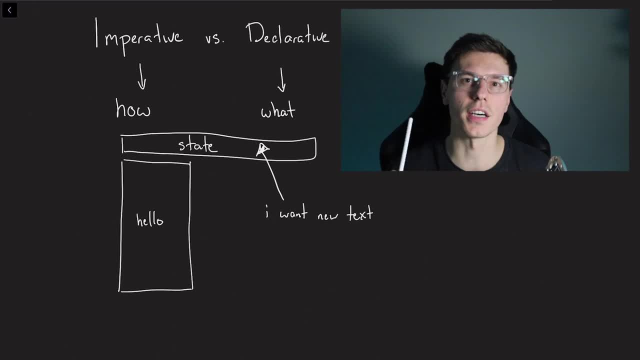 to change the text. Here we're saying we want to see a different text. it might seem like a small difference, but actually ends up being a pretty big difference when developing. I wanted to show you this in a real world example. So here we have an array of seven numbers And let's say: 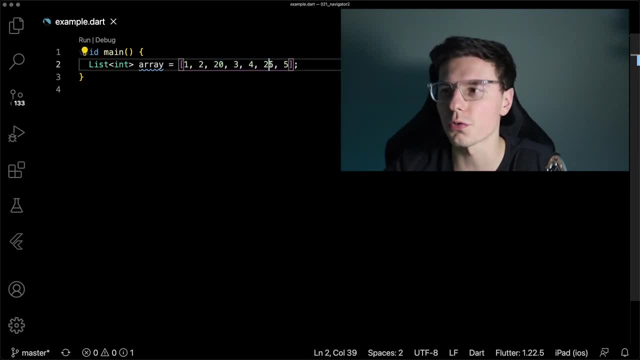 we want to remove all the numbers that are above 10.. You see the number 20 and 25.. But pretty much want those removed. So this is what the imperative solution for that would look like: shows you how to actually do this. First, let's define a new list that we want, with an array called array less than. 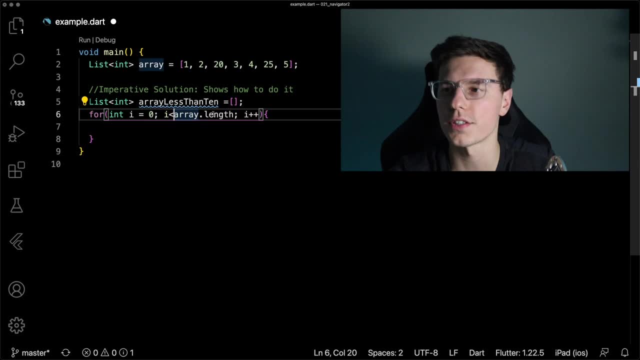 10. And then we'll create a for loop that goes through every single item in the array. Then we check each element if it's less than 10.. And then add that element into the new array that we have. then afterwards we're going to print that array. you can see, this solution tells exactly what the 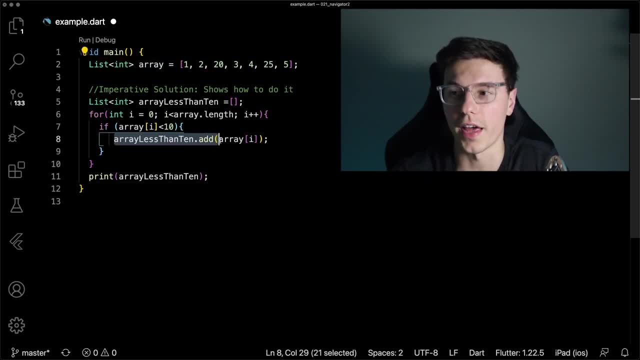 computer needs to do: go through every element and add it to a new array and then print it out, and we have the declarative solution where you pretty much tell the compiler what you want to see. So here we can start right away with the